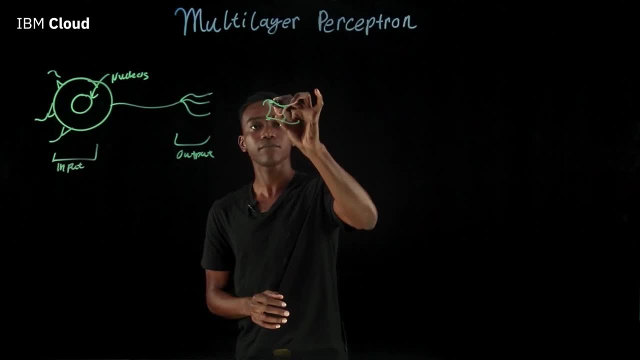 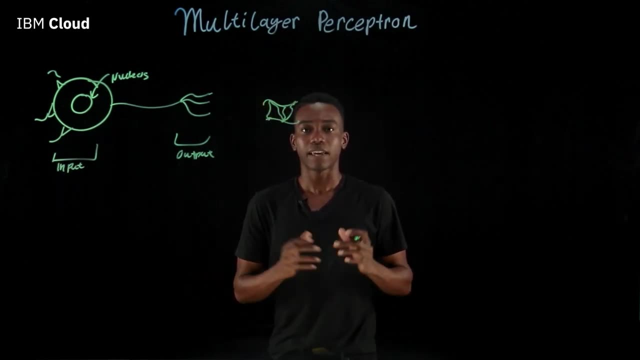 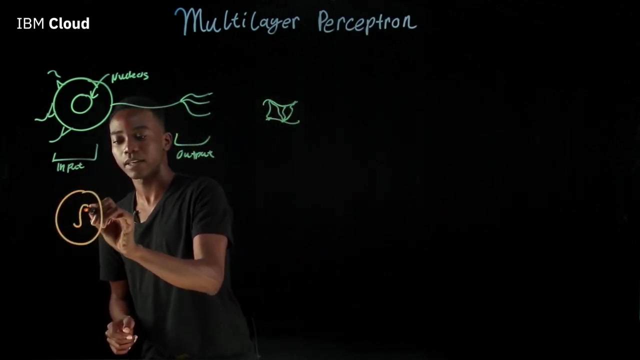 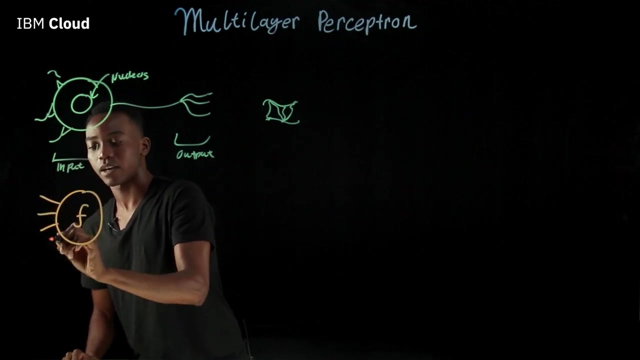 all working together in concert to get you the images and things that you see. In the same way, a perceptron is formed of three basic components. There's the function, which is the thinking part of the perceptron. There's the inputs that come in from other perceptrons. 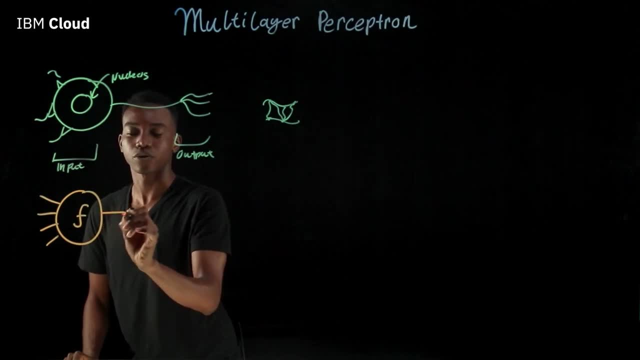 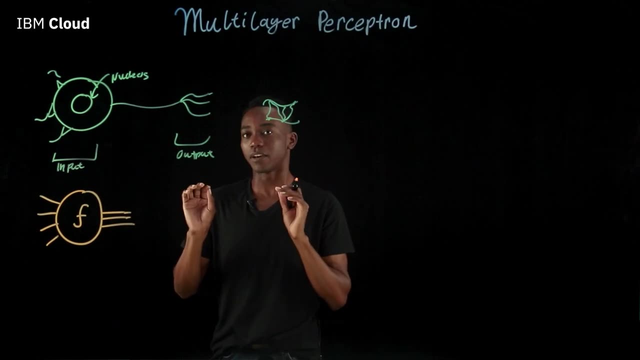 And, just like the neuron, there's also a set of outputs that go out from the perceptron. You won't be able to find a perceptron, It's just a concept. But the way that the perceptron is organized is also very similar to the way that our neurons are physically organized. 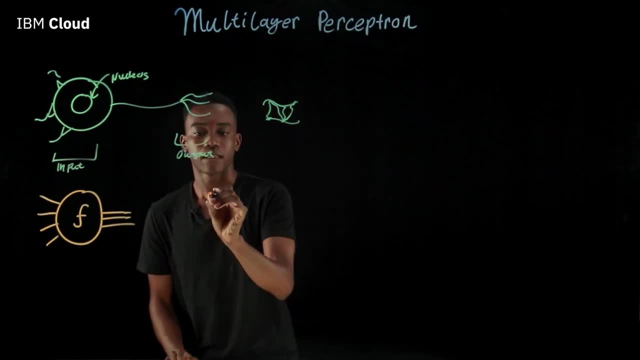 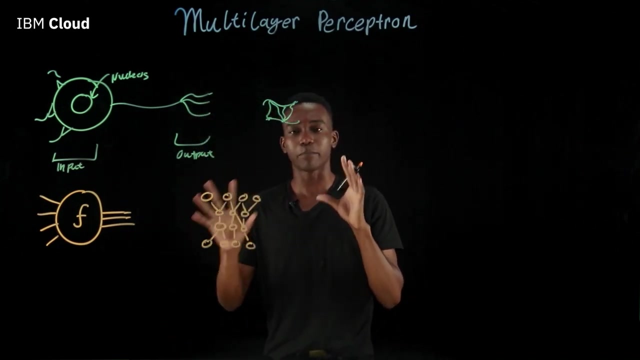 Perceptrons are organized in layers And this is where the multi-layer part of multi-layer perceptron comes in. They're all connected and they all feed off of each other's inputs and outputs. So this is just the basic concepts behind the multi-layer perceptron. 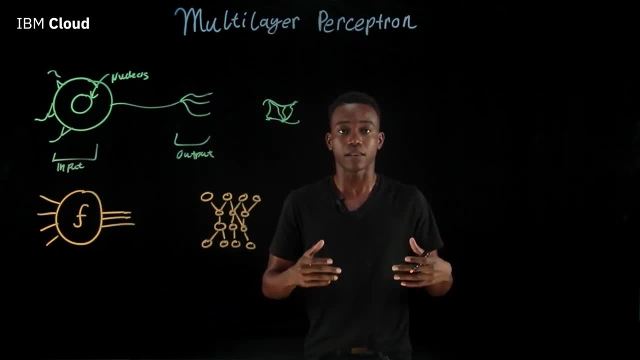 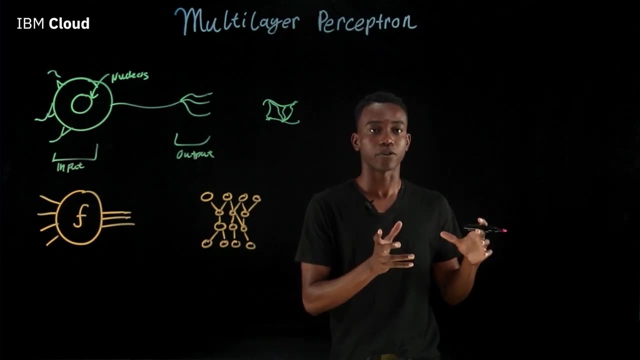 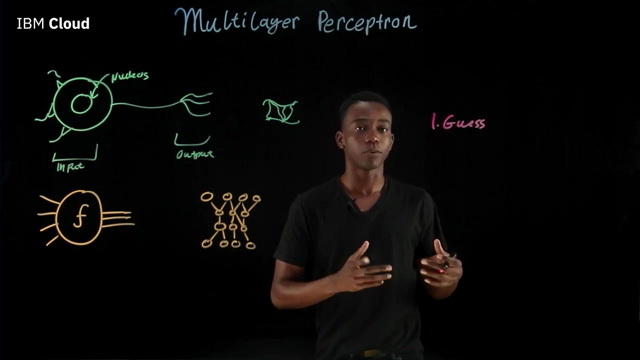 You're probably wondering how we do this, How we get computers to think and how we get multi-layer perceptrons to learn. Well, there's three basic parts of learning. First of all is you make an educated guess. For example, when you were learning four-legged animals, you would have seen a bear. 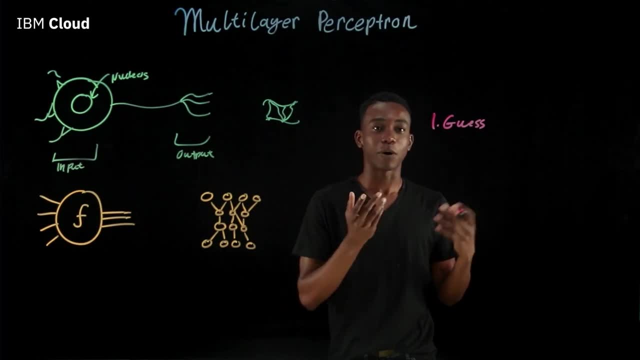 and you might have called it a dog. Why would you call it a dog? Why would you guess a dog? Well, dogs have four legs and a tail, and this particular bear has four legs and a tail. Well, you were wrong. 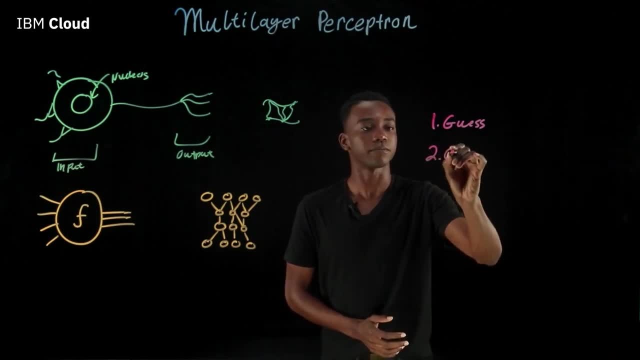 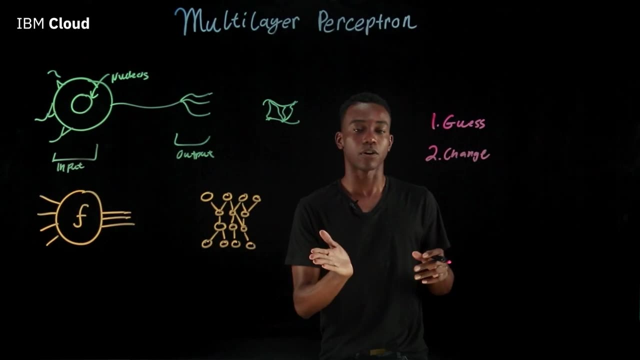 So what you have to do now is the second step of learning, which is to change. So you change your mind about what the difference between a dog and a bear, But what about the next time when there's a horse? Neither of those answers really work. 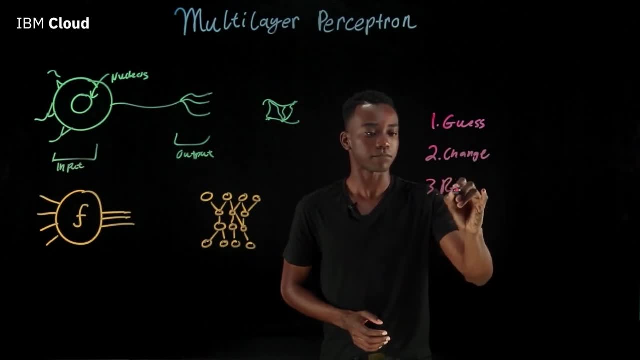 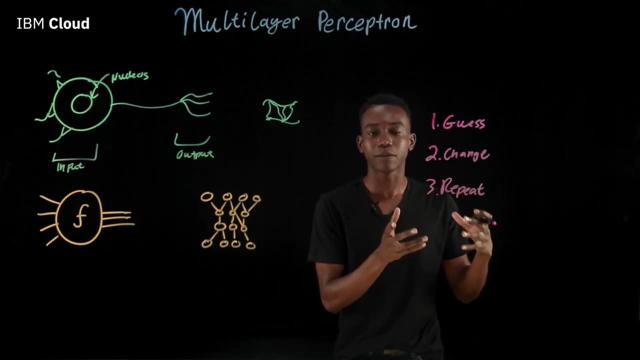 So what needs to happen is you need to repeat this process. This is basically the same way that scientists are able to train multi-layer perceptrons. First of all, the multi-layer perceptron gives an output Based on the function, based on the inputs, it gives out an output.